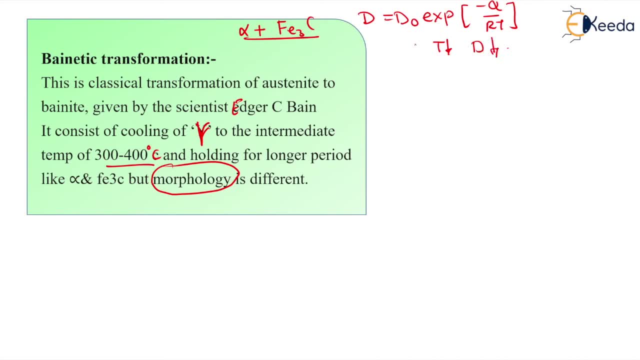 the diffusivity is also sorry. temperature decreases. As temperature decreases, the diffusivity also get decreases. So, dear students, again this is dependent on the diffusivity of carbon. Okay, So here, dear students, we are having at around 400 degree centigrade, we are going to get this upper bainite. 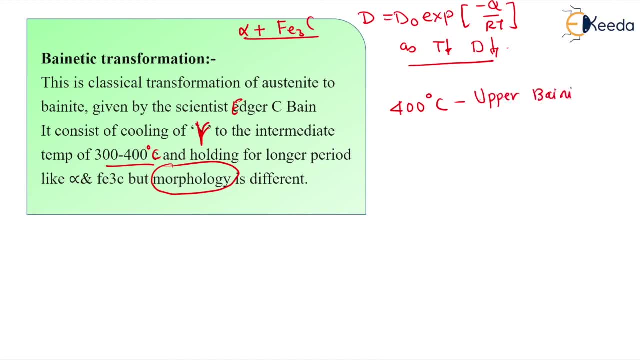 Upper bainite, Okay, And at around 250 degree centigrade, dear students, we are going to have this lower bainite, The lower bainite. So if we talk, dear students, see at this 400 degree centigrade, at this temperature, the carbon can diffuse significantly. 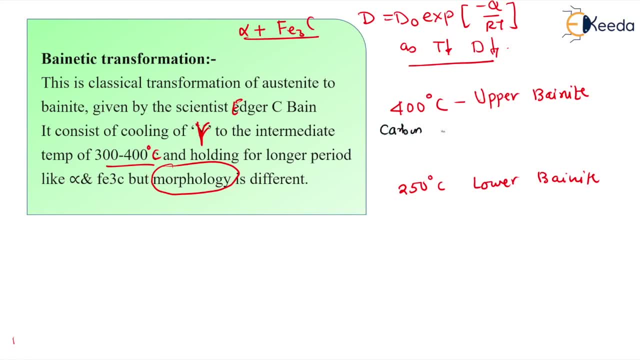 Here. this carbon can diffuse significantly, See, but this iron cannot diffuse, See, but this iron cannot diffuse, Isn't it So? but I will write here, but the iron cannot diffuse, And say: this bainite is known as the upper bainite. 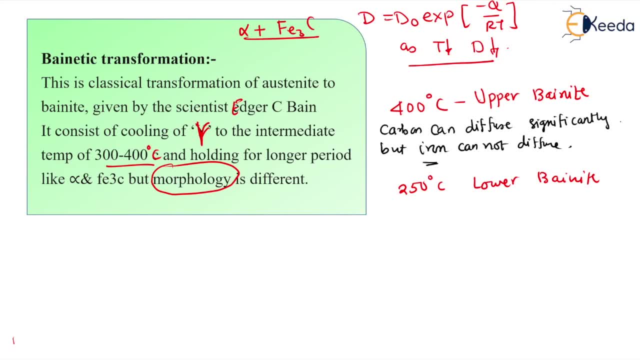 Okay, And the bainite at 250 degree centigrade. that is known as the lower bainite. So, dear students, let us now consider- I will consider here this lower bainite, Okay. So, dear students, when the transformation is going to occur at the lower temperature, say: I am talking about this 250 degree centigrade lower bainite we are talking about. 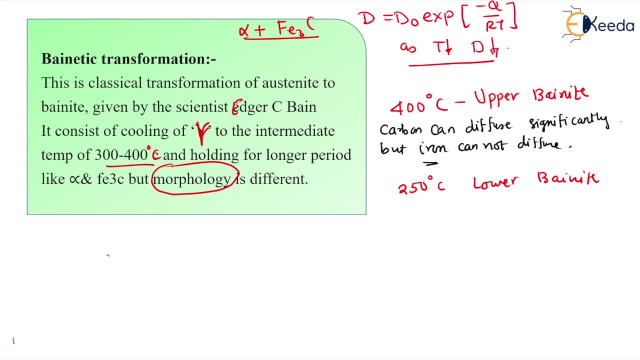 So this austenite will transfer, like say this gamma austenite, at say again, I am taking at this 950 degree centigrade And I am cooling down to say 250 degree centigrade. 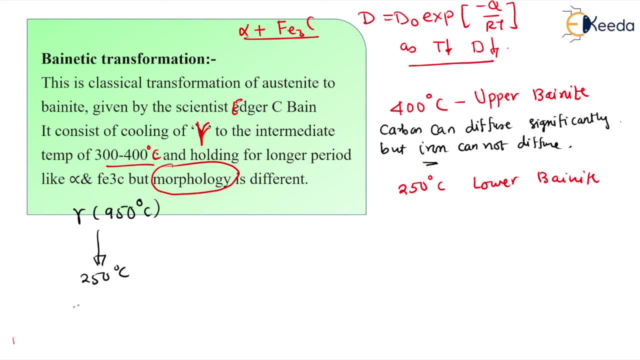 Okay, So it will get converted into dear students. at 250 degree centigrade definitely the alpha, But this alpha is dear students, the supersaturated alpha. Alpha is how The supersaturated alpha. So how the supersaturated alpha actually. 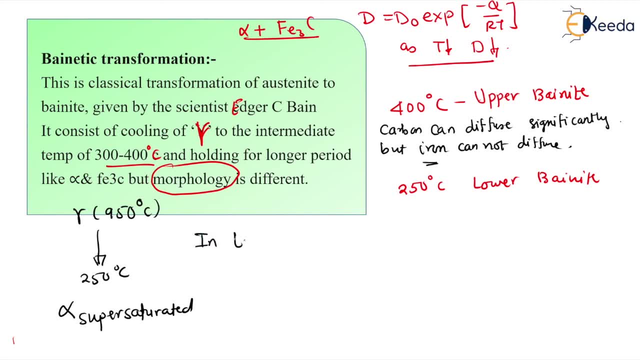 In terms of the supersaturated, in terms of, in terms of the carbon, The supersaturated in terms of carbon, dear student, But, dear students, at lower temperature, At lower temperature. So BCC iron will not take, will not take any carbon. 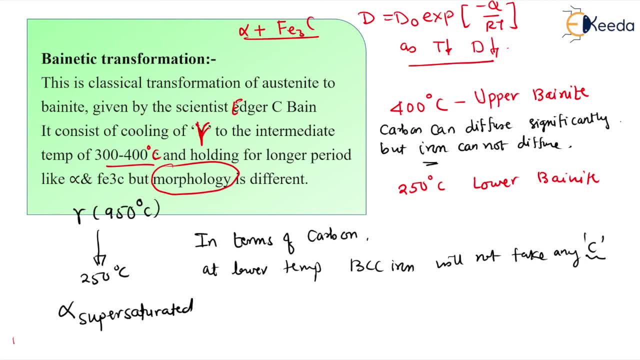 So actually, this is the pure iron, isn't it? Below this, below 727 or at, say, 250 degree centigrade, This BCC iron, alpha iron, is not going to take any of the carbon, isn't it? 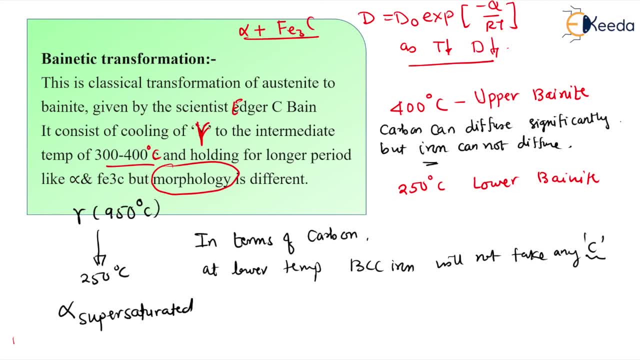 And that is the reason why it is supersaturated. Okay, So it will not going to take any carbon at that temperature. So what will happen, Therefore? so it get precipitated as the cementite within the supersaturated alpha. 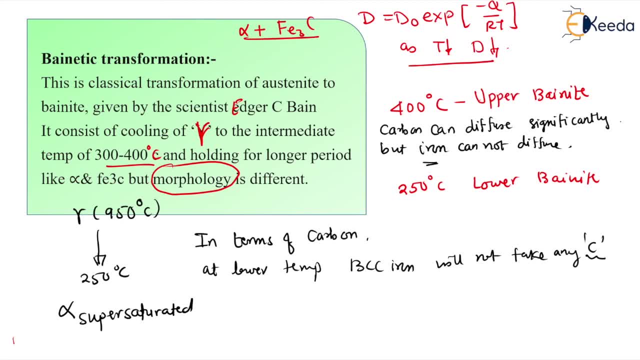 So what happened here? So definitely this alpha is the supersaturated In terms of the carbon, because at lower temperature this BCC iron not going to take any carbon, So therefore this carbon is going to precipitate as the cementite within this supersaturated alpha. 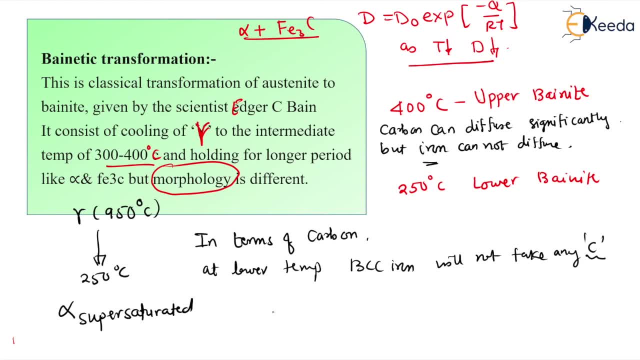 Okay. So if I say this is the supersaturated alpha, If I draw here, say this is the supersaturated alpha, So within this supersaturated alpha The carbon is going to precipitate like the cementite. The carbon is going to precipitate like the cementite. 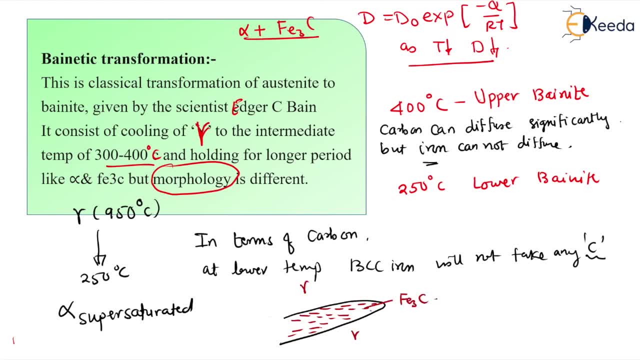 Okay, And say: this is the gamma here. This is the gamma. We are cooling down to the 250 degree centigrade And we are going to have this alpha supersaturated- Supersaturated in terms of carbon, Okay, Okay. 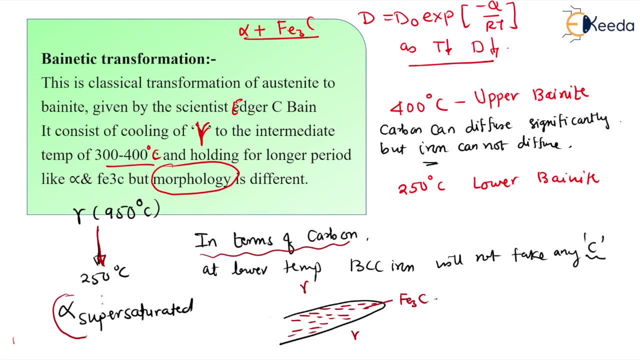 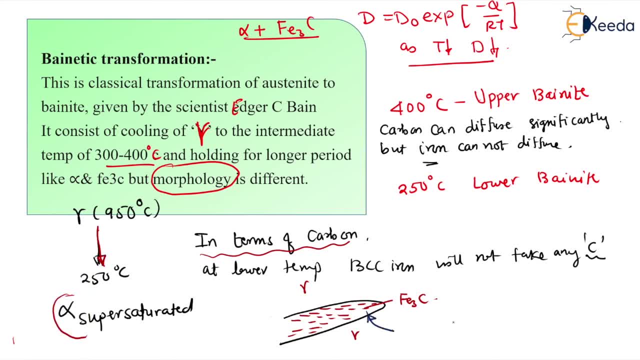 This is our supersaturated alpha. Okay, I will show you. This is our supersaturated alpha, Okay, Okay, So this is how This lower bainite is going to form, dear students. Okay, And this alpha, which is supersaturated, comes like the woodman's statin plates. 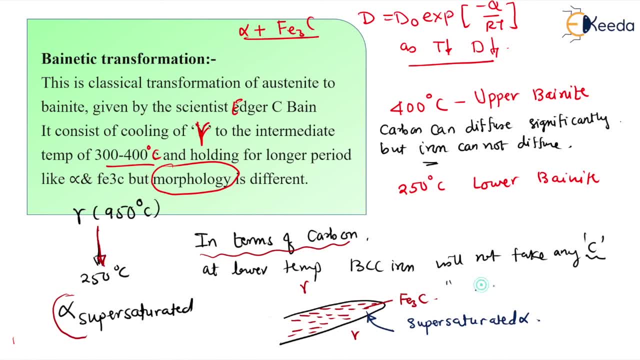 Okay, How it is. look like It is the woodman's statin, Woodman's statin plates. Okay, Which is having the two morphologies or only one morphology? It is look like the sheath, Okay. Okay, The morphology is what? 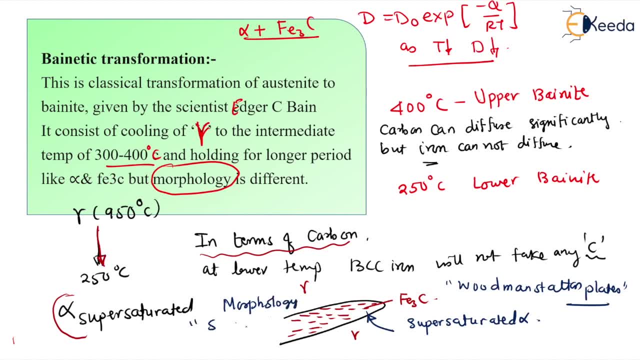 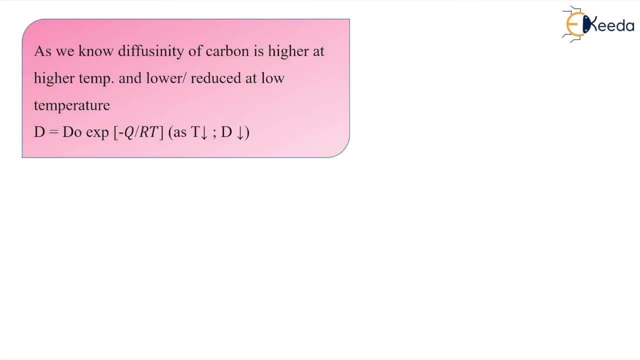 Is the sheath? Okay, Talwar is like that shape, Okay. So this is about the lower bainite, dear students, And if I talk about the upper bainite, dear students, If I talk about the upper bainite, 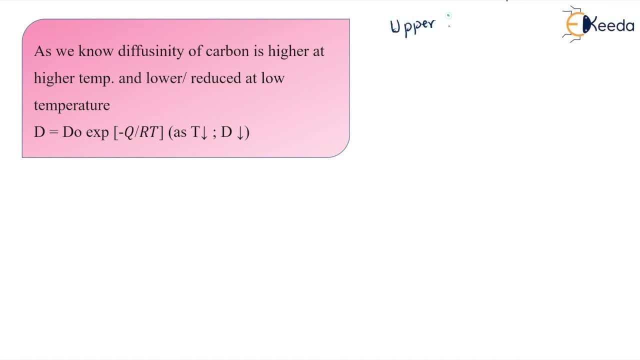 Upper bainite. we will discuss now, So in the slide. So the upper bainite is going to be like this. So the upper bainite is going to be like this. Okay, So we will see. 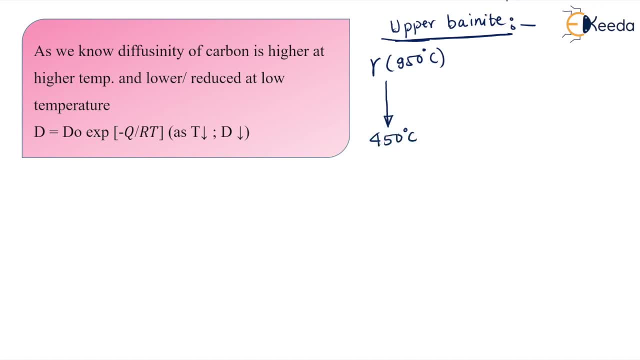 So the upper bainite is going to be like this. Okay, So here. so in between this alpha and cementite, sorry, in between this alpha, in between this alpha, the cementite get precipitated, get precipitated. 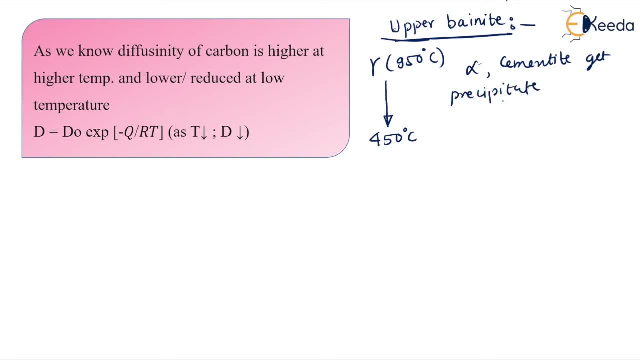 So where will this cementite get precipitated? Between the space of these alpha plates? So I will draw here. Okay, so these are all the alpha plates, These are all alpha. So here this cementite is going to. 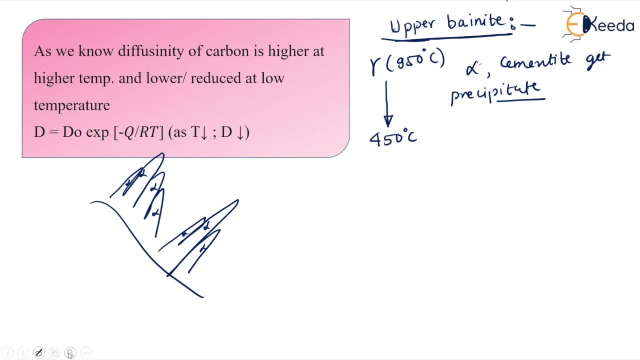 precipitate between these plates. So I will show with the red color how it is precipitated between these alpha plates like this. Okay, so this red precipitation is all. So this is how the upper bainite is going to form, dear students. 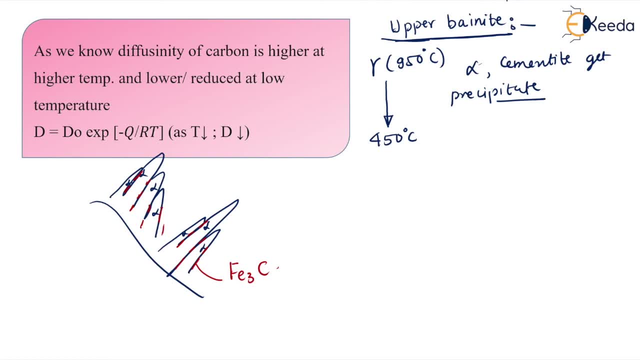 So, if you look at the thickness of these plates, which are very less okay and strength will be very high and ductility also very good for this. So, dear students, so there is one method, chemical method or process which can reduce this thickness of this cementite. 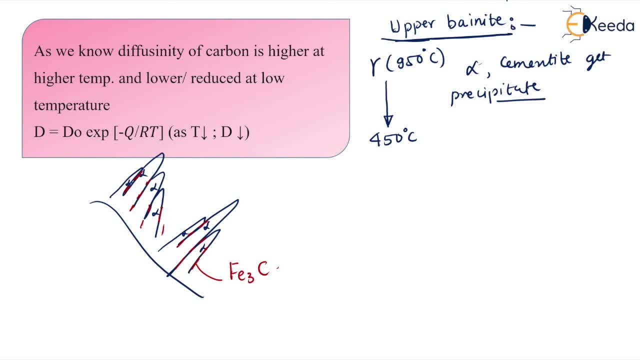 So if you look at this metal material, we will find that if there is enough silicone bias between these plates, that means we can convert this thickness of this cementite which precipitate, which is precipitated between this alpha plates. that is, from we 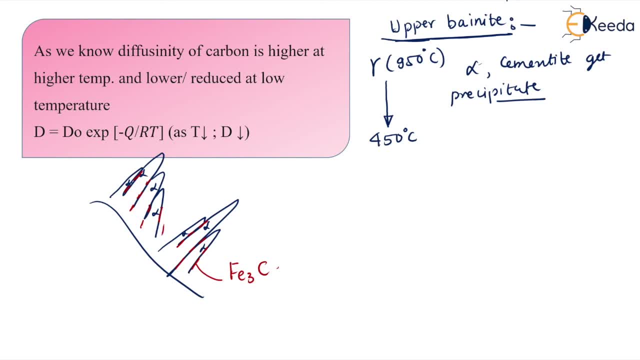 So if you look at this metal, so this metal which is precipitated between this alpha plates, that is, from. we can convert this thickness of this cementite precipitates from this micrometers to the nanometers Programme for Chechen De promotions from this micrometers. 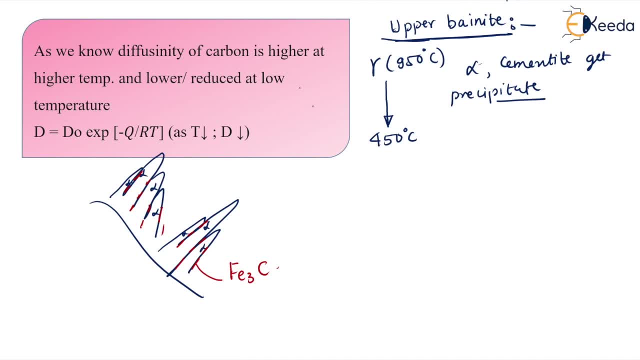 to the nanometers, micrometers, and it was discovered by the Harry of longer from Cambridge University, from Cambridge. Dear students, there are very less industries in this world which are going to form the, actually the bainite, which are used in the industrial applications or used Only. 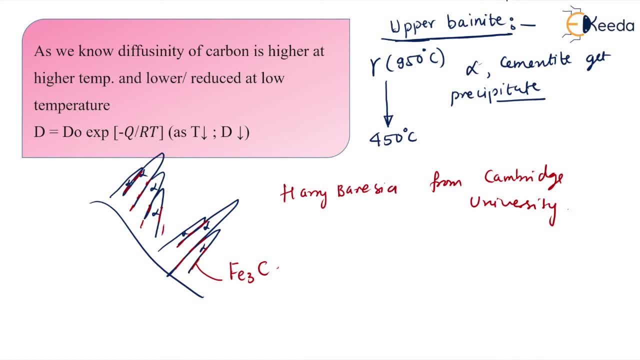 one steel manufacturing or steel producing industry is there, that is, the Bosco steel plant in the Korea where this bainite is generally used or produced for the industry use. So there is only one steel plant, that is the Bosco Bosco steel plant, which is in Korea. 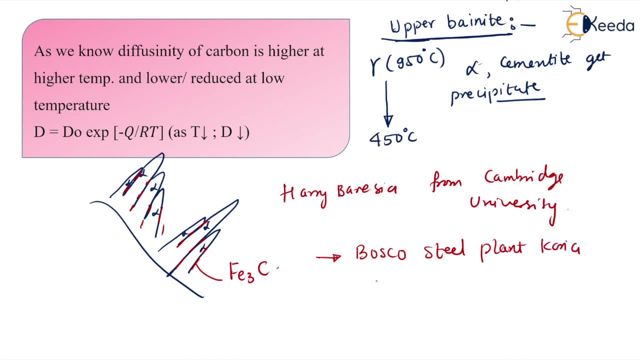 is going to produce, or they are producing, this bainite for the industrial use, for the industrial use. So this is about the bainite, dear student. Still, actually, we not have the confirmed literature for this bainite, but some of the literature where they mention this bainitic transformation. 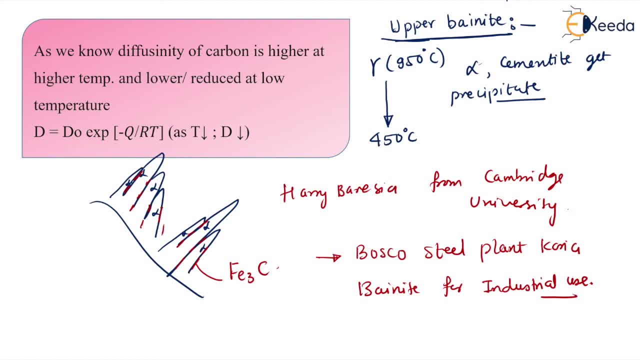 is like this way, Isn't it? And especially, it is given by this HRC Bain. That's why this transformation is known as the bainitic transformation. So here we are having the two types of bainite. The first type is the bainitic transformation. The second type is: 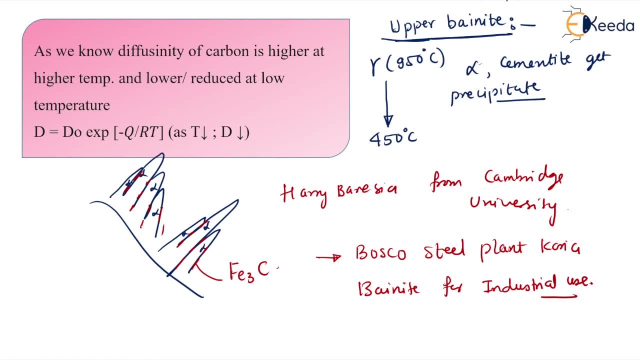 the bainitic transformation. So here we are having the two types of bainitic transformation. So here we are having the two types of bainite. dear students, When we cool this gamma austenite to the 250 degree centigrade temperature, this is the lower bainite which is having. 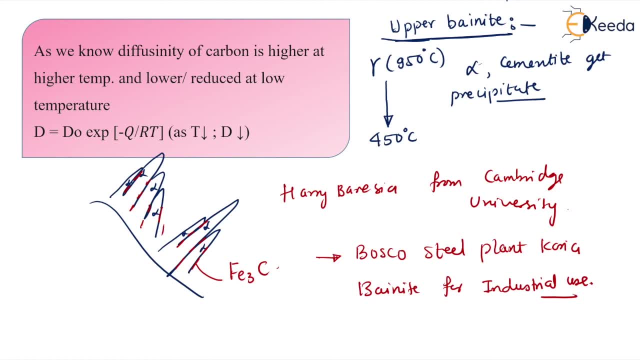 the sheath like morphology. And, dear students, at around 450 or 400 degree centigrade we cool the gamma austenite. So this cementite is going to get precipitated between the plates of the alpha, Isn't it? 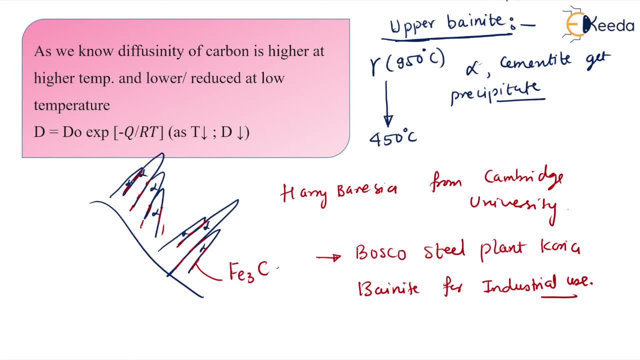 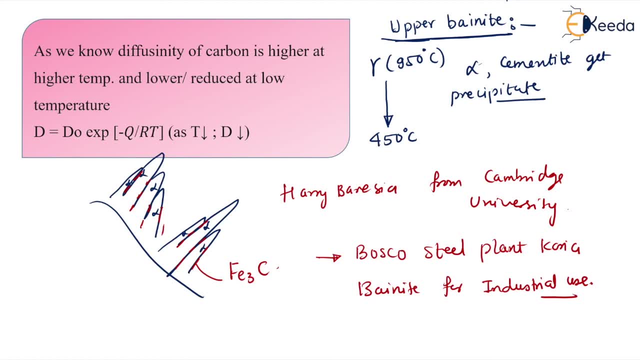 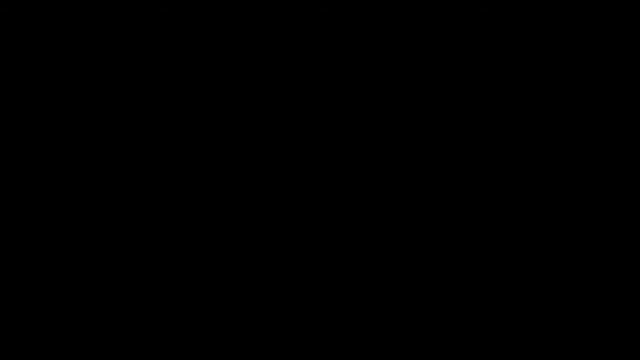 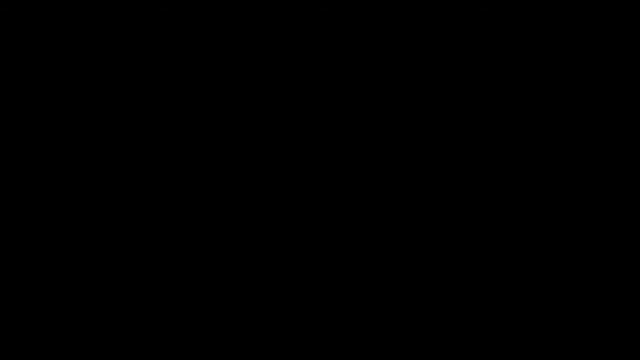